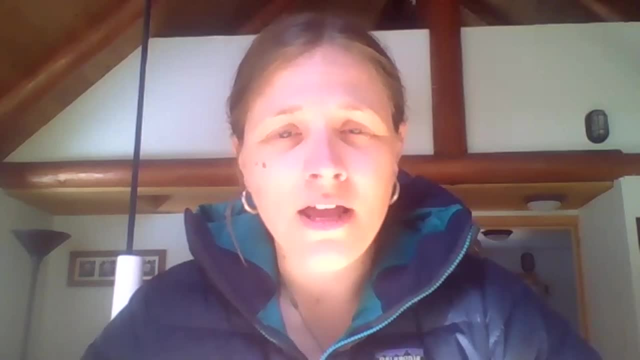 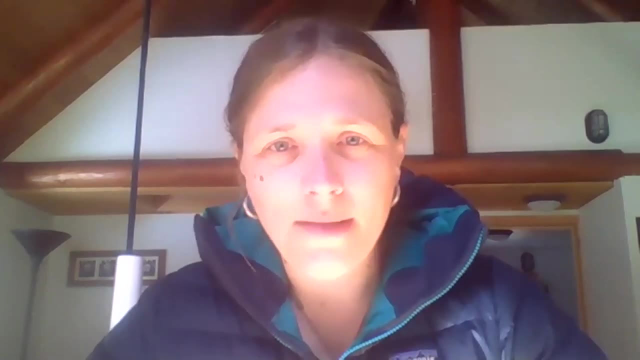 planet, And then I'm going to skip to the end of the chapter and talk about, or near the end of the chapter and talk about the arid or kind of dry climates of the world, And then I'll talk about the other climates in the next section. just to break it up, So let me share my screen with you. 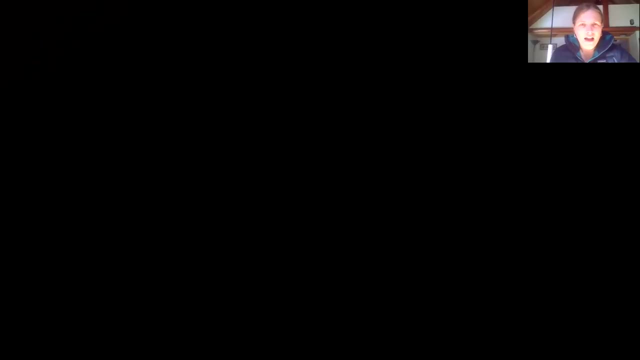 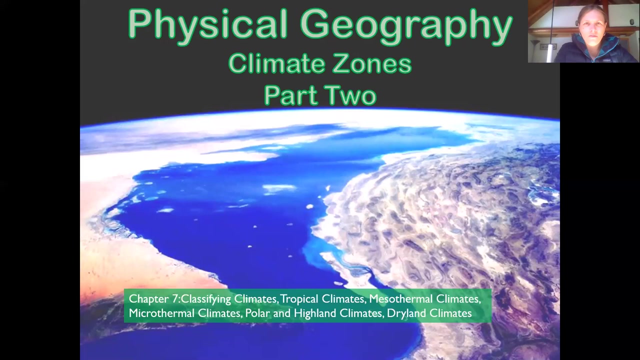 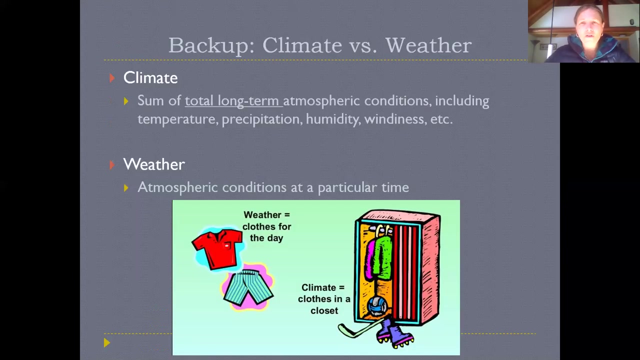 here. Okay, Oh wait, let me go back. That's the second part. Okay, So again, this is chapter 7.. And I already kind of told you the sections that we're going to talk about. So when we think about climate zones, I want to first make sure that everybody understands what. 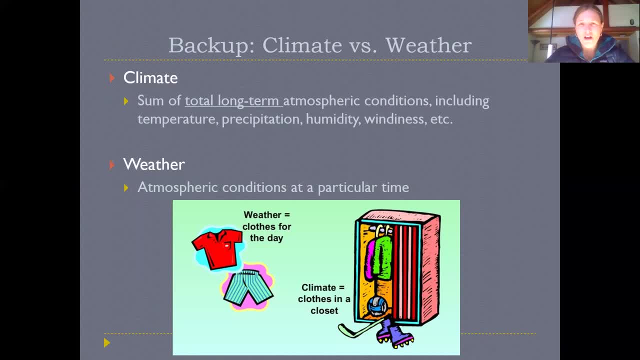 climate is, And so climate is often kind of used synonymously with weather, And while they are related, they do have differences, And so climate is the total long-term atmospheric conditions that exist in a particular area. So these atmospheric conditions include things like: 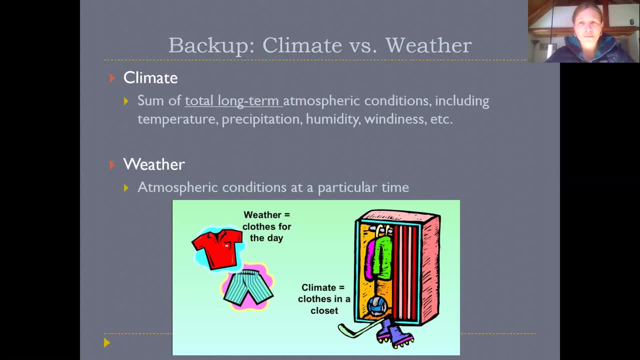 temperature, precipitation, but also things like humidity and windiness, and so it's kind of a total phenomenon of what's going on with the water or what's going on, sorry, with the air, but not at a moment in time, but kind of continuously over time. 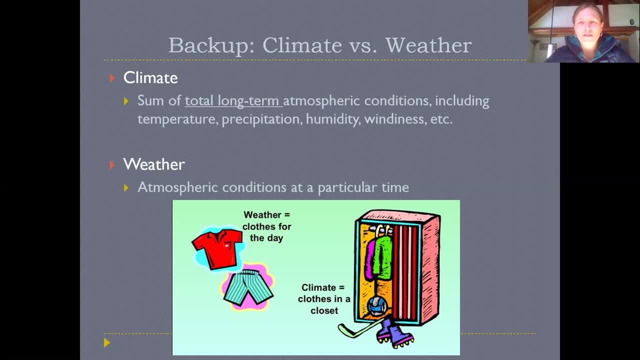 kind of a bigger picture, Whereas weather is what's happening at a particular moment. So the weather is what's happening this afternoon, whereas the climate is what exists there over years or decades. So sometimes the analogy is used like what you're wearing this afternoon. 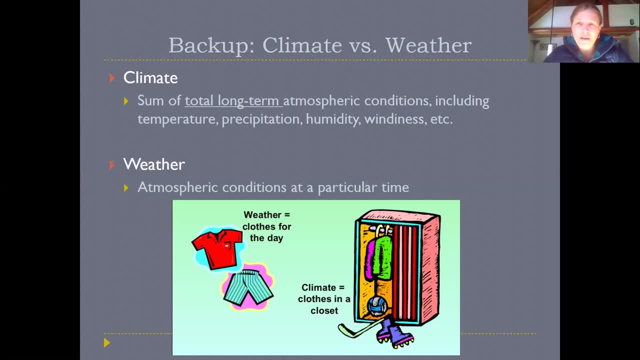 maybe is a raincoat, Rain jacket and long pants, or maybe as a tank top and shorts, whereas the climate is more like your closet. To exist and survive in this location, you need to have a warm jacket and you need to have a t-shirt, because it's going to get hot later in the year, And so if you're an organism that 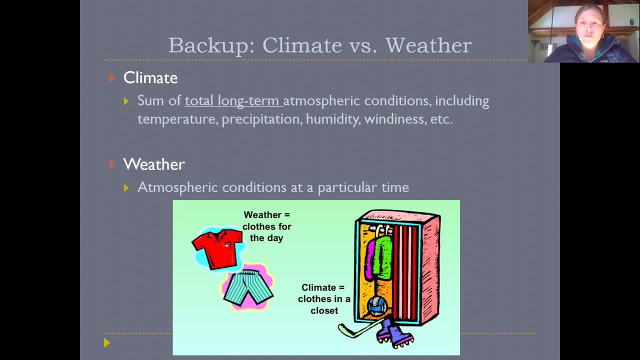 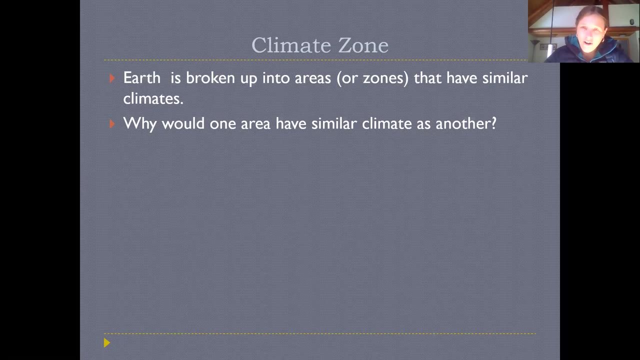 lives in a zone, you need to have kind of the tools to deal with all the different kinds of atmospheric conditions that could exist within that area's climate. So this chapter in particular talks about climate zones. So a zone, of course, is an area. 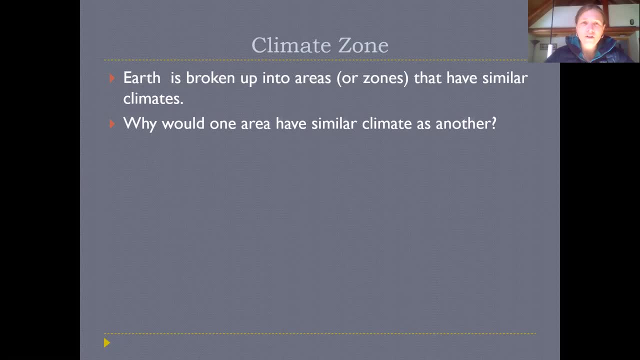 And so what a climate zone is is a zone within the earth that has a certain climate, And so the earth has been broken up into many areas that have similar climatic conditions. So, as we just said, that means similar temperatures, similar precipitations, similar windiness, similar 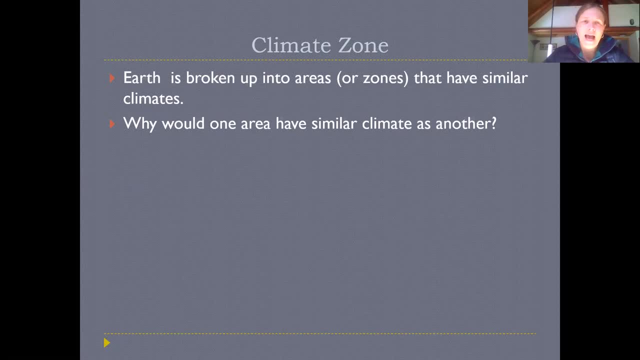 humidity, seasonality, And so the climate zone is a zone within the earth that has a certain climate. So we have already, throughout the semester, spent a lot of time thinking about what are some of the things about the solar energy, about the seasons, about the way that storms might move wind and 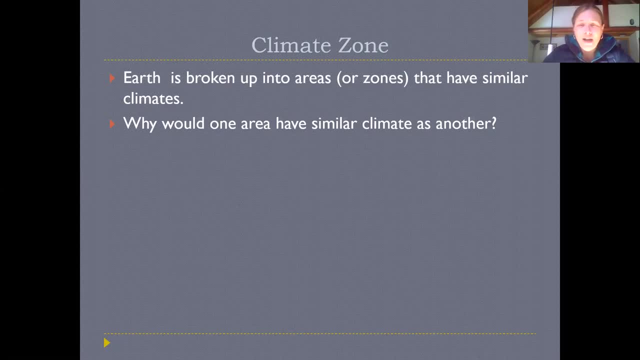 rain might occur in different areas. that would impact why different areas in different parts of the world might in fact have similar climates. So I would encourage you guys to maybe pause this video for a second and do some brainstorming, See what you can think about, And then we'll. 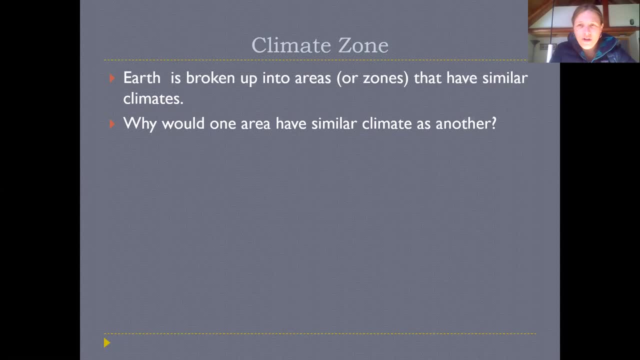 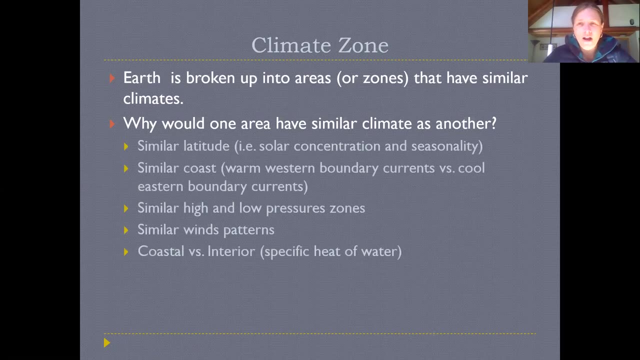 see what you can think of, But let me share with you now that hopefully you've paused and done that. here's some of the things that we've talked about so far. that might cause different areas, perhaps in different hemispheres- right, one area in the northern and one area in the southern. 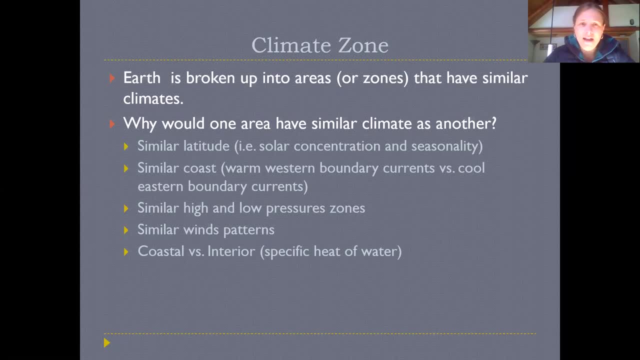 or in different continents, one area in Asia, one area in America, to have similar climates. So one would be latitude. We know that different areas of latitude have different amounts of solar radiation. So we know that different areas of latitude have different amounts of solar radiation. 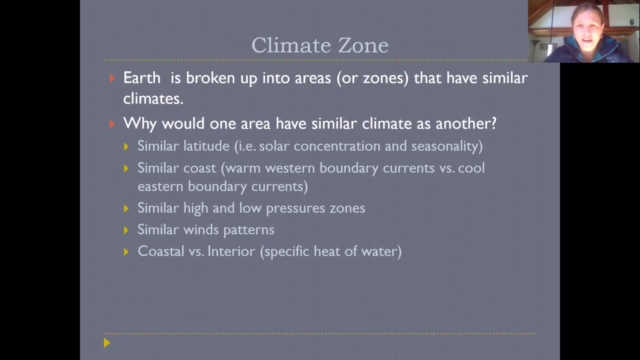 hitting them, essentially because of their angle relative to the sun. They also experience different seasonality. We've talked about how being on an east coast or west coast influences the kind of ocean currents that you're exposed to, which might affect humidity of the air, and 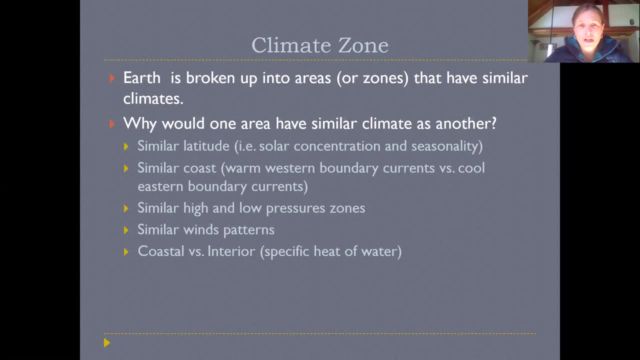 then eventually precipitation and raininess in certain zones. We've talked about being in high and low pressure zones and that, how that higher pressure zones tend to be drier And lower pressure zones tend to be kind of stormier zones. And then we've, more recently, 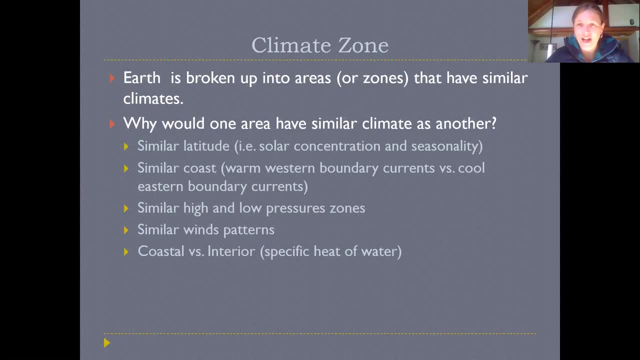 learned about that. we have these different kinds of fronts- frontal uplift, convergent uplift- different kinds of things that might cause precipitation in these lower pressure regions. We've also talked about wind patterns, And then we've also talked about the influence of specific 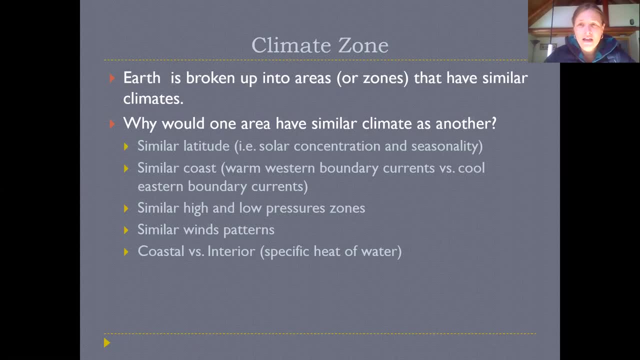 heat in climate. So being close to a big ocean in a coastal area is going to make you feel like you're going to have a more moderate climate. right, Because the ocean is absorbing stealing energy from you in the summer when it's hot, and then slow releasing that energy back to you in the 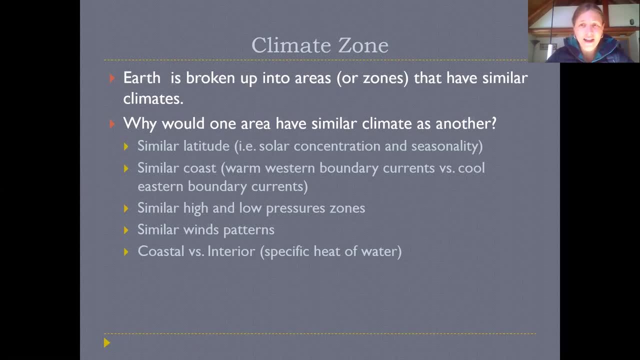 winter, when it's cold and keeping you more mild than in an inland area. So hopefully those are some concepts that you feel good about so far, And now we're going to kind of think about how these different things come together to make different parts of the world have different 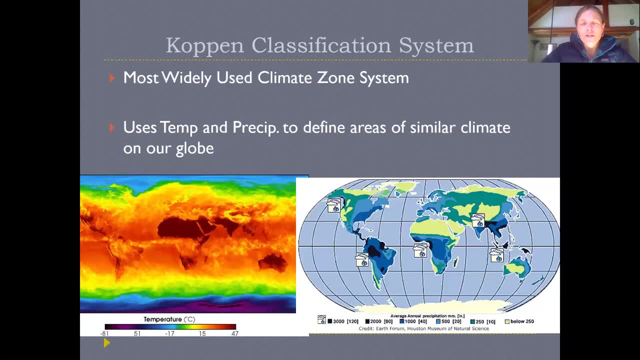 types of energy. So we're going to talk about how these different things come together to make different parts of the world have different types of climate. Okay, so there's different ways that we have classified or broken the earth up into different zones with different climates, But kind of the most. 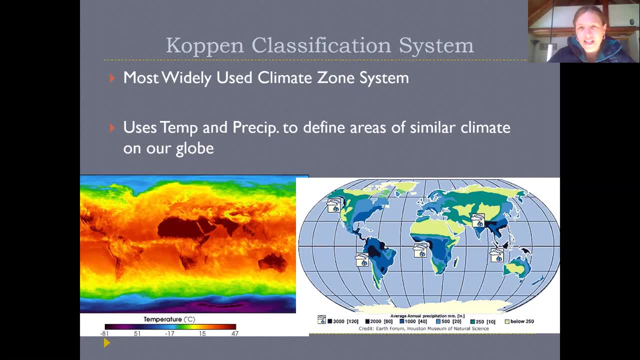 standard, widely used system today is called the Copin classification system. It's been around, I think, for about 100 years And it basically uses two main, very important climatic characteristics: First temperature, So the bottom left image shows different temperature areas, And then 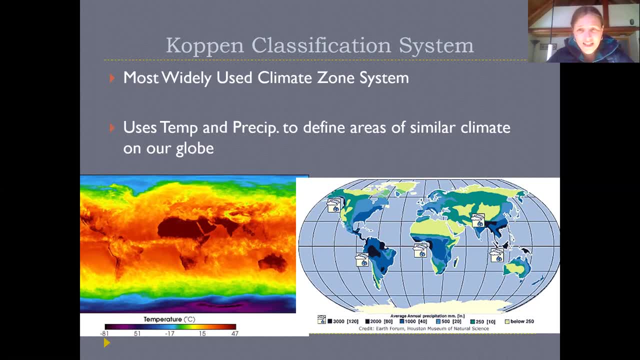 precipitation, And not only amount of precipitation, as this map in the bottom right shows, but also seasonality of precipitation that we talked about in the last lecture, And it kind of combines these two factors- ranges of temperature, ranges of precipitation- to break up the world into these. 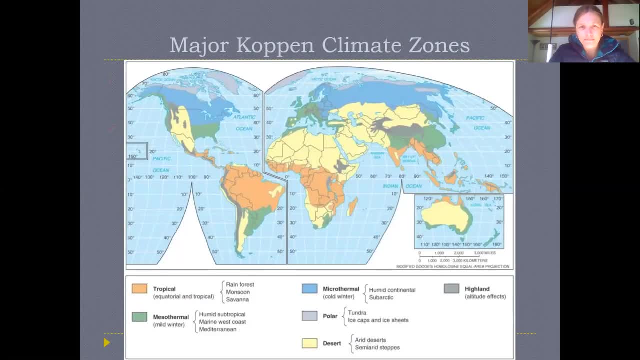 different areas that share similar climates. So here is a map with kind of a simplified Copin climate map Over the earth, And so in this case, it's showing us six different colors or six different zones, The first one being the tropical zone along the equator in orange, The second one being the mesothermal zone, which is 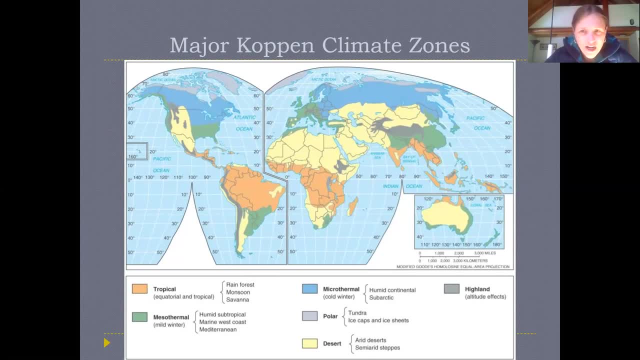 kind of a middle meso meaning middle, thermal meaning temperature, kind of a moderate climate zone, in green That's where we live, Blue a microthermal- micro meaning small, thermal meaning temperature. so a very cold, low temperature zone up in kind of Arctic regions, or not quite in the Arctic, but high 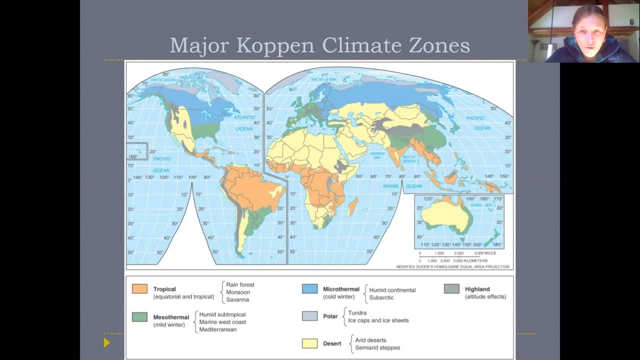 latitude regions, Polar all the way up at the poles, in light gray And then yellow, being desert zones. These are zones that are kind of defined by their extreme lack of water during large parts of the year, And then finally there's a slightly darker gray color. that's for highland climate. So these are kind of high mountain areas. 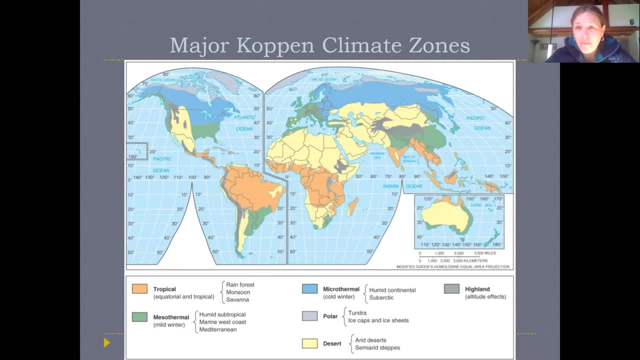 And, as we've already learned before, the higher we go up in the troposphere the colder it gets, And so those highland areas actually have quite similar climates to polar areas that are quite cold during most of the year. So we can see that the earth can kind of be broken up into these different zones that share different climates And so 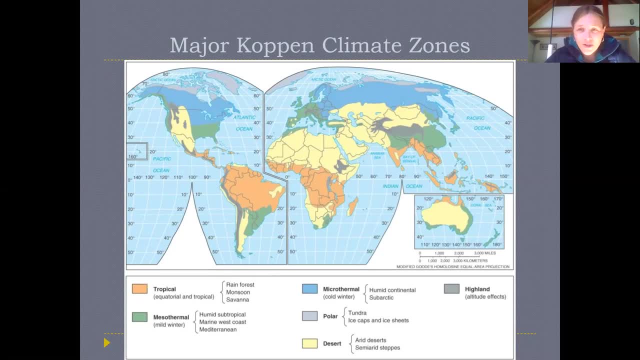 therefore, the organisms that live in these different parts of the world are going to have to have similar adaptations. they might look similar to each other, they might even be similar to each other or actually be exactly the same from one continent to another. 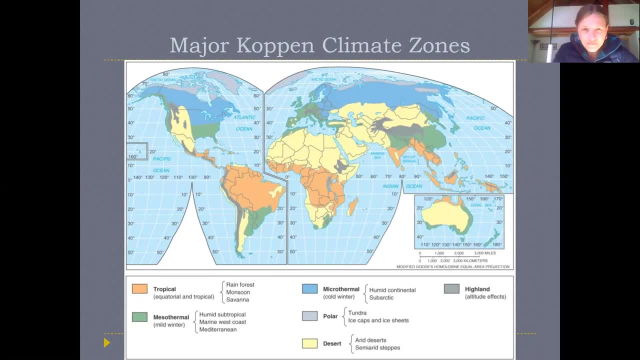 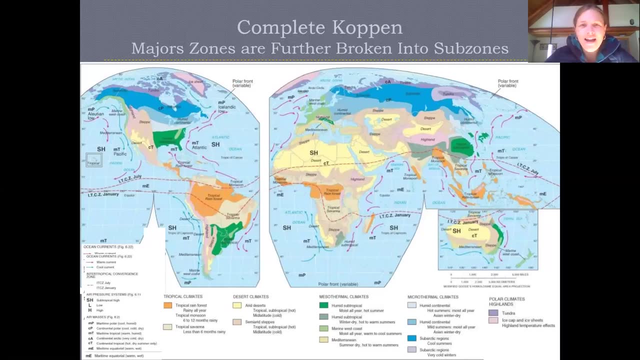 And that's because of the climate there. So of course scientists don't like to leave things just nice and simple, But the Copan system breaks up each of those bigger zones: the tropical zone, the mesothermal zone, the microthermal zone, the 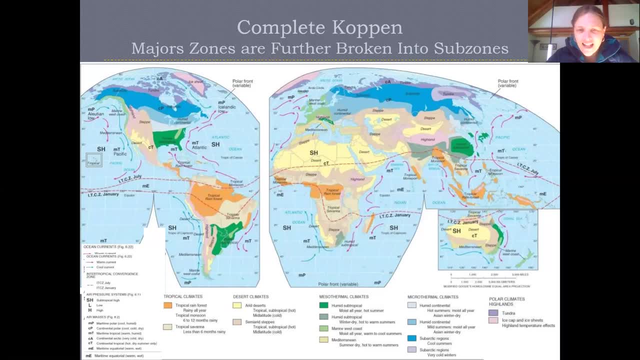 tropical zone, the mesothermal zone, the microthermal zone, the tropical zone, the mesothermal zone, the microthermal zone, the kind of desert or dryland zones, and then the polar and highland zones into kind of further categories. So this is kind of a more. 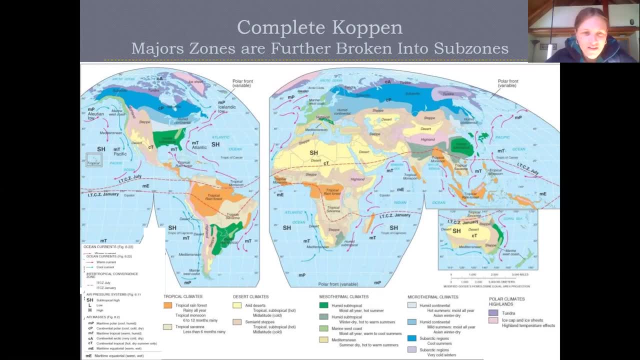 complex world map that shows within the tropics there are more extreme wet areas and then there's more seasonally hot wet areas and the dry climates have the extreme dry and the less dry areas and mesothermal climates have different climates with some more seasonality and 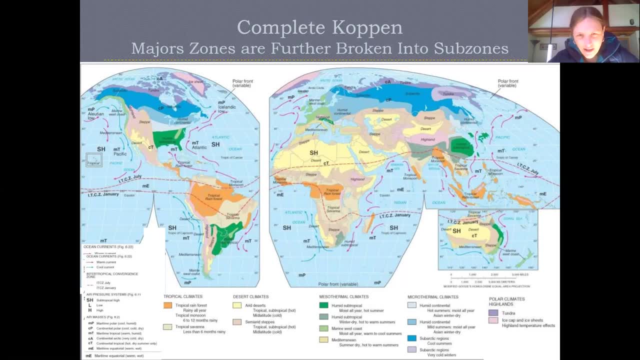 precipitation variables, etc, etc. So this map also shows some interesting kind of some of the high and low pressure zones that we've drawn on our global map, So our SH standing for subtropical high pressure zones, And then it also shows some movement of different kinds of air masses and that might be moving into different areas. it 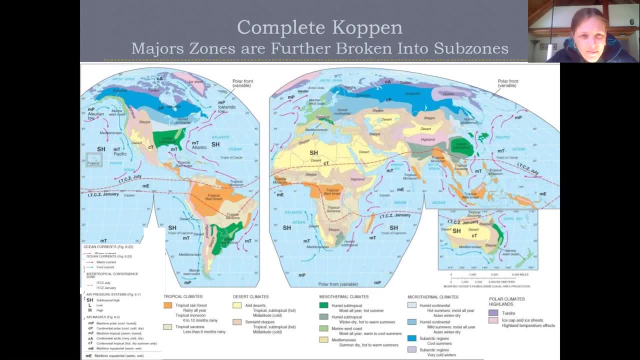 shows warm and cool ocean currents and purple and blue And the ITC and the ITC Z zone, that intertropical convergent kind of equatorial weather zone. So again, this is kind of layering a lot of the information that we've already learned about global patterns into this. 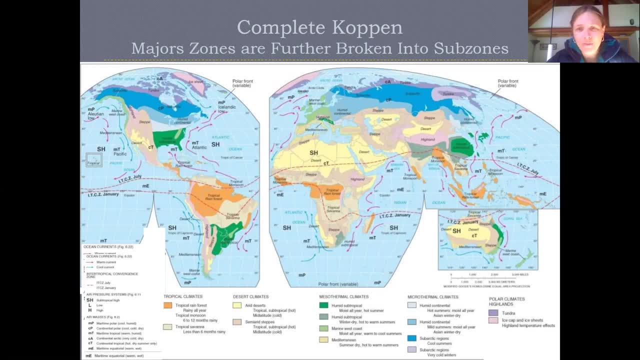 picture of what the climate is actually like in any specific part of the world. So we're going to go through and kind of look at some of these zones and talk about some of the names that we would give them and talk about some of the more specific characteristics that they have. And then when 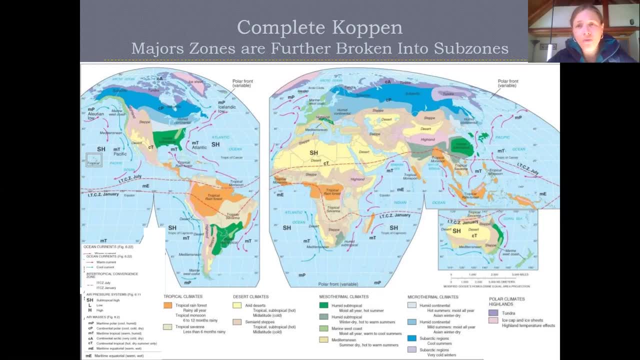 we're done with chapter seven. we are going to actually jump all the way ahead towards the end of the book to chapter 16, which talks about global biomes, which are basically different kinds of ecosystem communities, And so we're going to kind of think about why different kinds of 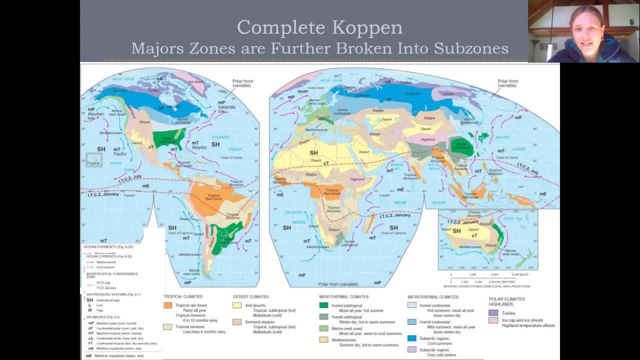 plant and animal and other organismal communities might exist in these different climate zones, But we're not there yet. I'm just kind of giving you a framework for where we're going. Okay, so first of all, we'll start with the major coping climate zone that's called the humid. 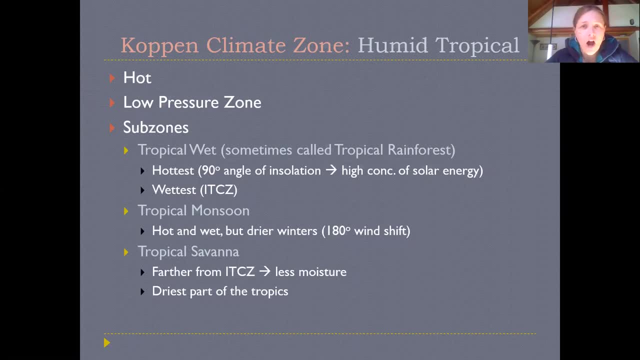 tropical zone, So this is the hottest part of the planet. We know the equator already is at extreme low pressure zone, So it's continually pulling air in. The trade winds are continually converging on the intertropical convergent zone. They're experiencing convergent uplift, So they're 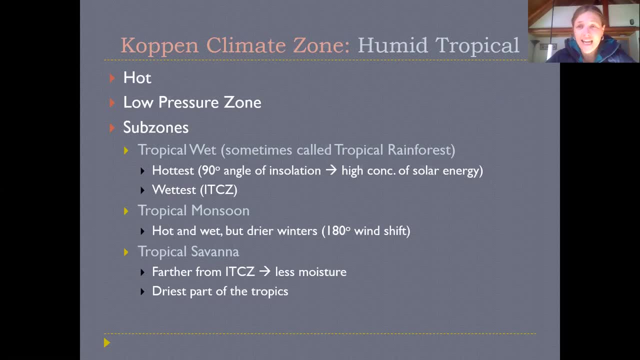 rising And then they're experiencing adiabatic cooling. right, They cool as they rise up, which causes clouds and rain. So this is not only a very hot but also a very rainy part of the planet. But within the tropics there are some differences, So there's one part of the tropics 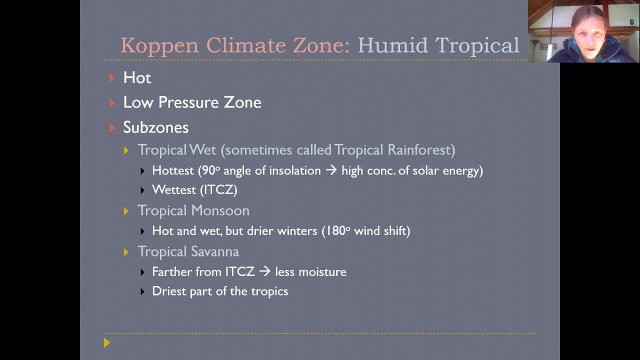 that's called the tropical wet or sometimes called the tropical rainforest zone, And that's the hottest, wettest part really right on the equator, right on that intertropical zone, Tropical convergent zone. Then there's a tropical monsoon zone. We've talked about how monsoons 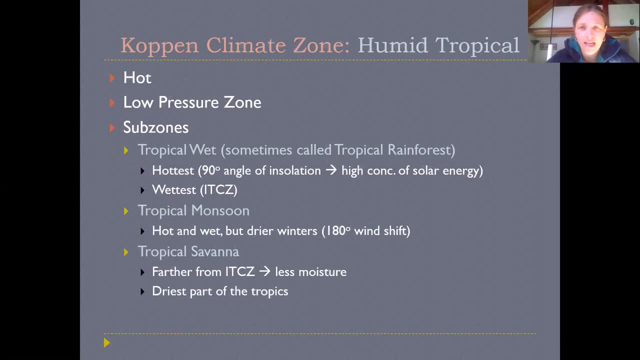 work, basically these complete shifts in areas near the equator where the ocean is meeting the land- Okay, so that creates these seasonal differences. And then the tropical savanna is an area that's a little bit farther away from the equator, kind of approaching the subtropical. high pressure zones, And so you know it's a little bit farther away from the equator. And so you know it's a little bit farther away from the equator, And so you know it's a little bit. 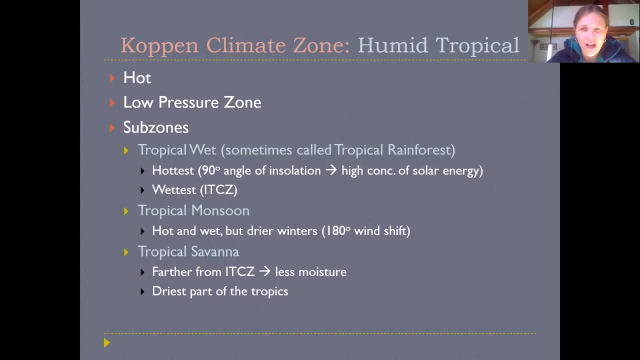 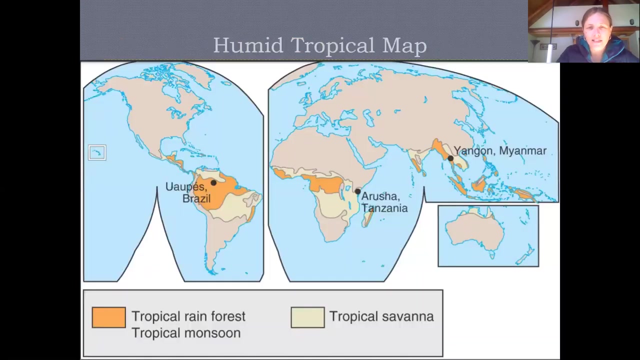 it experiences some tropical climate, but also a little bit drier and more seasonal, a little bit more like the climate of a subtropical high pressure zone which, we'll find out later, is more of a desert type of zone. So let's kind of look at some maps. So first of all, 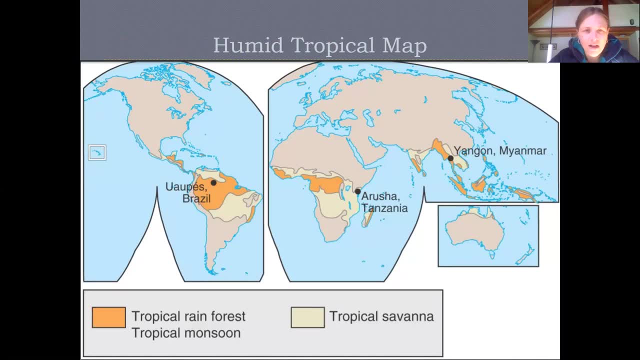 this is showing the humid subtropical area And the areas in orange are the rainforest and the monsoon, the wetter areas. So that's like the Amazon Basin, the Congo Basin in Africa, Indonesia, these areas that are really wet And, as you can see, they all kind of line up along. 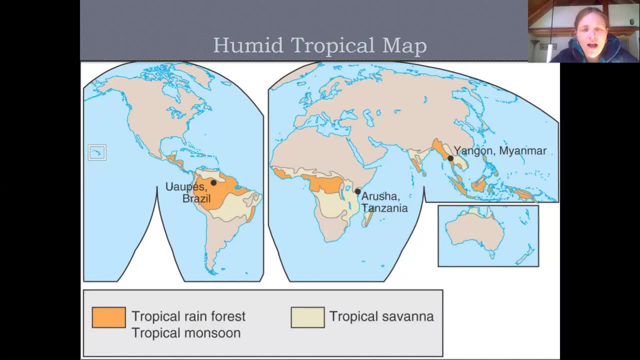 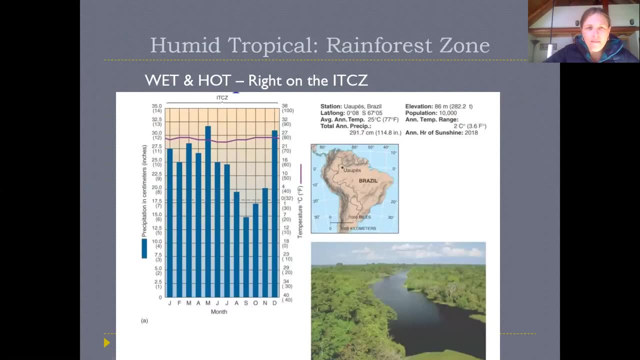 the equator And then we can see in yellow kind of farther afield from the equator there are these tropical savanna zones. So first of all thinking about where a rainforest zone might exist- Again, this would be like very close to the equator. There's a little map on the kind of upper right. 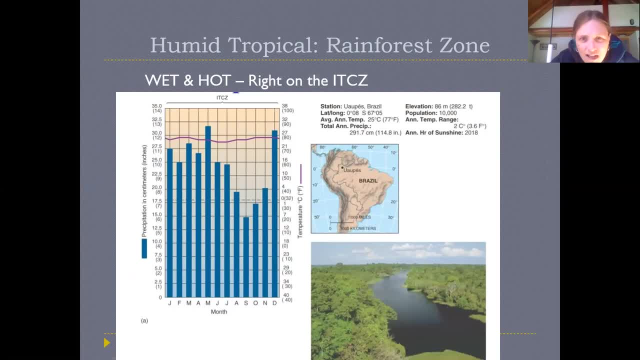 showing Brazil and showing this particular town in Brazil, which I'm going to pronounce wrong, but you can see it's right on that, zero degrees latitude. You can see below it's a rainforest, And then you can see in the graph on the left that all during the different times of the year. 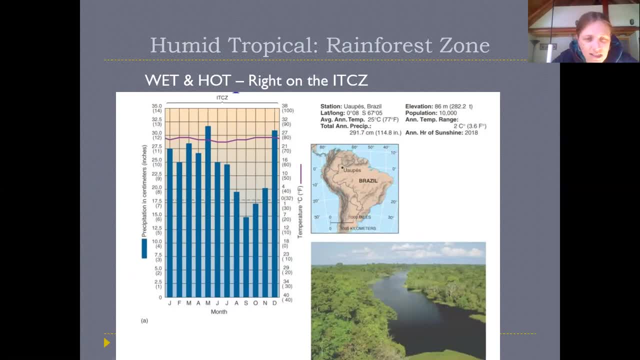 there is significant precipitation, So some months have might have less than others. the lowest month has 15 inches of precipitation. the highest month has more like 30 inches of precipitation. But keep in mind that parts of Southern California get less than 15 inches of precipitation in the whole year. 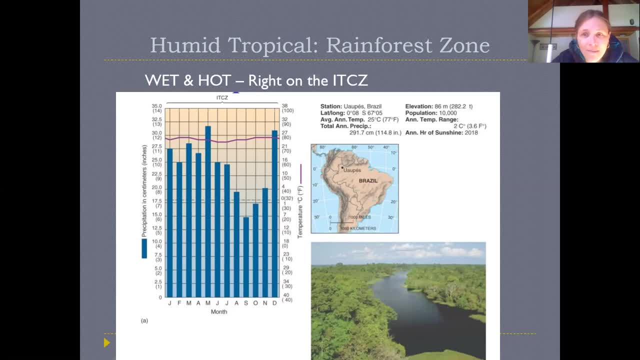 And that's how much rain this area gets in its lowest month, And so this is a very rainy, rainy, wet part of the world. And then, as we'll talk about when we get to chapter 16, this is going to kind of influence the ecosystem. 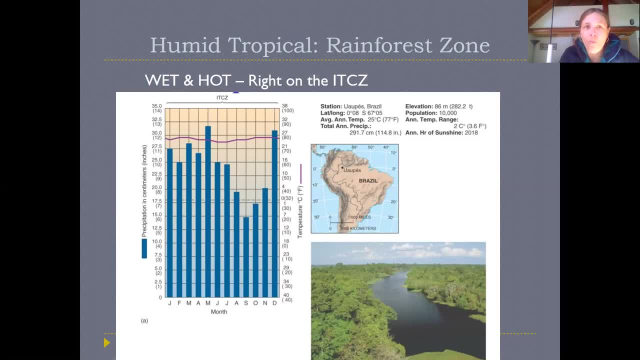 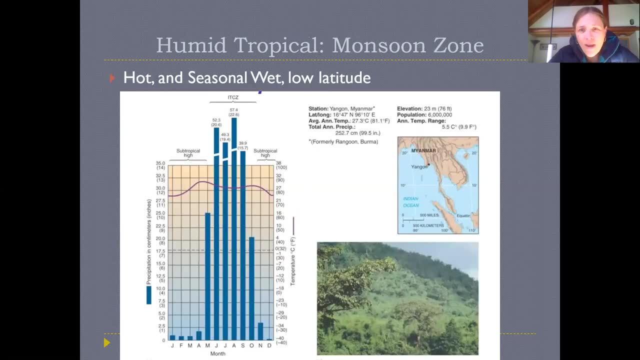 the kinds of organisms that are able to live here. So wet, wet, hot, hot right on the equator. Okay, then we have monsoonal zones, And so, in this case, this is showing Myanmar, And, as we've already discussed before, monsoons happen when we have areas that are relatively 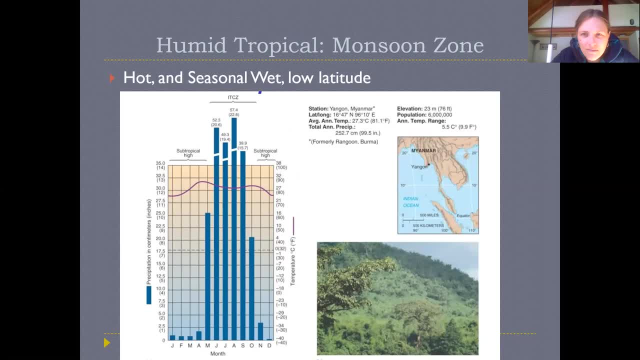 close to the tropics, And then they're usually where we have some sort of landmass that's oriented with an ocean below it, So like where we have a continent that's not really vertical up and down but kind of a horizontal continent, So like in Southeast Asia and India and like Texas. 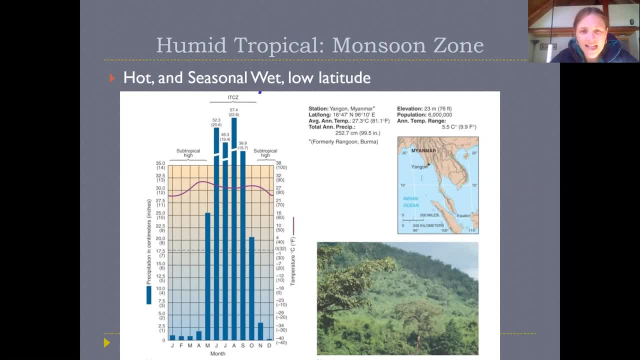 and Louisiana gets this a little bit too, And in this case we already talked about these forces before, but we have this kind of extreme difference in the seasonal winds that exist here, as we have these onshore and offshore breezes, but also kind of as the different 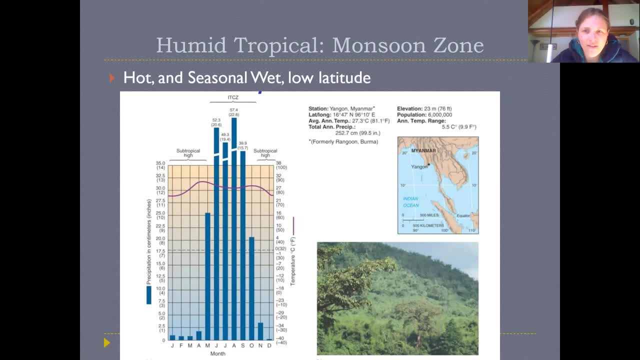 seasons occur, that particular part of the world kind of gets closer to the solar equator and then closer up to more of a high subtropical zone in their drier part of the year, which for them is their winter, And then their wetter part of the year is their summer, So again opposite from us, And this is the kind of thing. 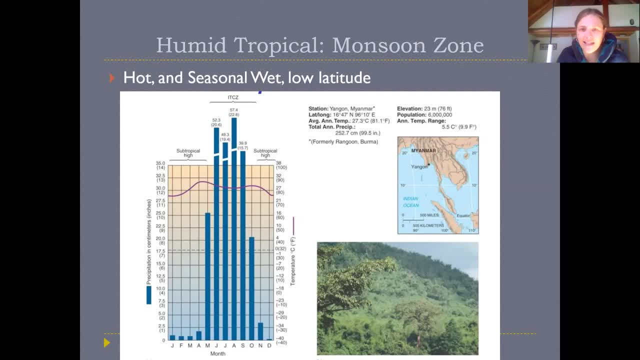 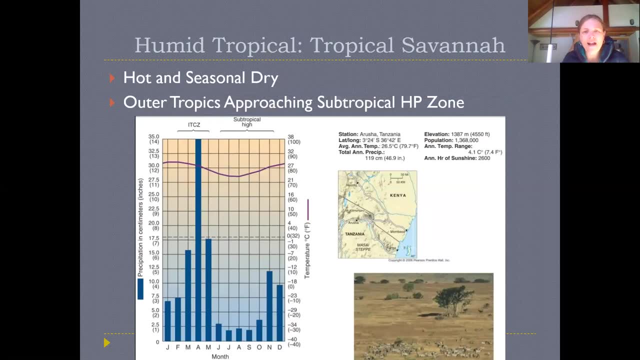 that's experienced again in India and in places like Southeast Asia. Okay, so then finally, we have that kind of most outer part of the tropics that are approaching these subtropical high pressure zones, So they spend a considerable amount of their year kind of having the high pressure system. 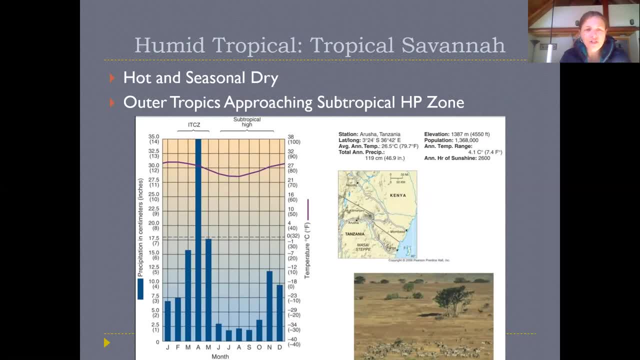 kind of block storms from coming in, And so they might have a short season, which is often in their winter, where they do get rain, but then they're going to have long dry seasons of the year as well, And this is going to cause much more water deficiency through parts of the year. 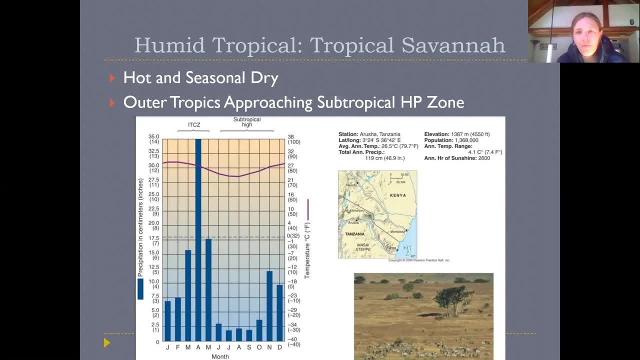 And so the vegetation is going to change a whole lot And we're going to have much more of a savanna, an open type of system, in places that we see, like in Africa, in the savanna in Tanzania or other places that you have kind of seen. classic African savanna type images. 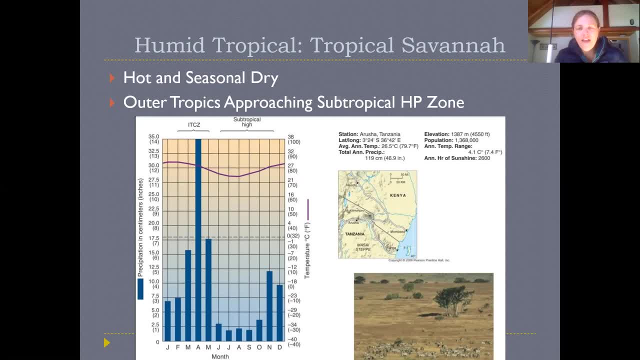 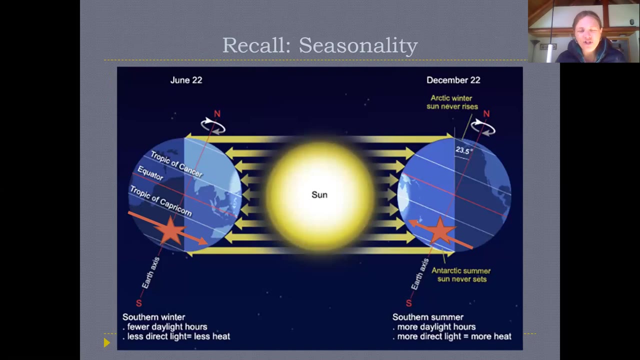 Okay, so this is a savanna type ecosystem. We don't only have these in Africa, we could have this in Australia, we could have this in South America as well, But this is the kind of thing that it would look like. Okay, so, as I'm kind of mentioning that in different times of the year, a certain area might be sitting closer to the subtropical high pressure zone and closer to the ITCZ kind of low pressure zone. 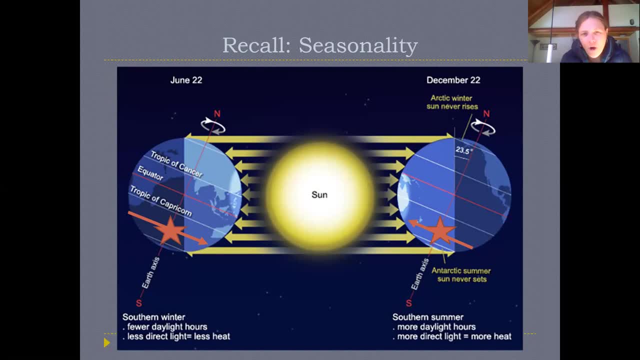 And I just want to kind of remind people how that might work. So before, when we talked about where there's low pressure and where there's high pressure, we kind of said that low pressure is always at zero degrees and high pressure is always at 30 degrees, And in fact that's a little bit of an oversimplification of what we see in reality. 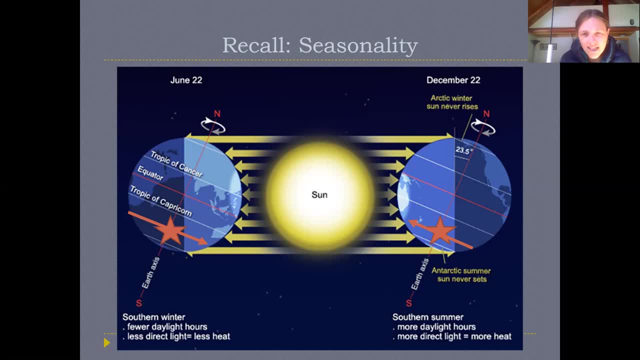 Because we have already learned that the Earth is tilted on its axis And as it moves around the sun, in different seasons, in different parts of the year, the sun is shining on the earth. And as it moves around the sun, in different seasons, in different parts of the year, the sun is shining on the earth. 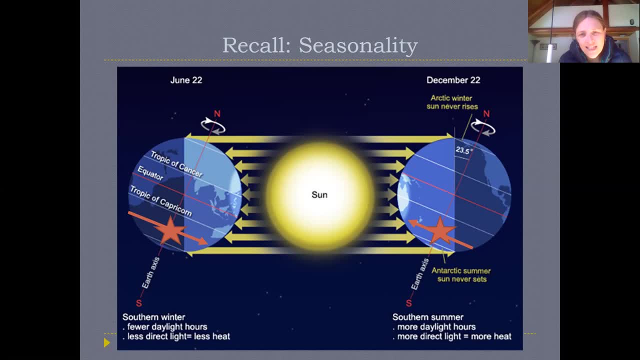